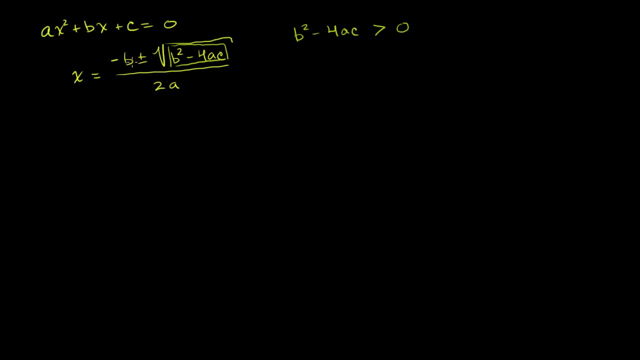 We're always going to have a b over 2a or a negative b over 2a. so you're going to have negative b plus It's that positive square root and a negative b minus that positive square root, all over 2a. 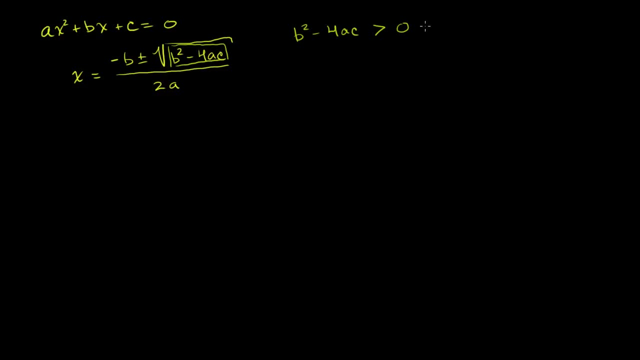 So if the discriminant is greater than 0, then that tells us that we have two solutions. Now I just used a word, and that word is discriminant, and all that is referring to is this part of the quadratic formula, That, right there. let me do it in a different color. 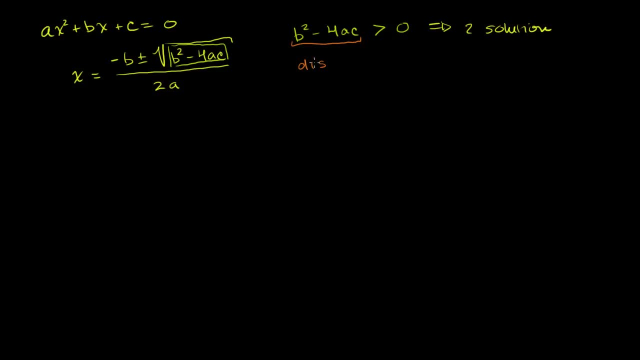 Right here is the discriminant, the discriminant of the quadratic equation, right here. discriminant, You just have to remember, it's the part that's under the radical sign of the quadratic formula and that's why it matters, Because if this is greater than 0, you're having a positive square root. you'll have the positive and negative version of it. you'll have two solutions. 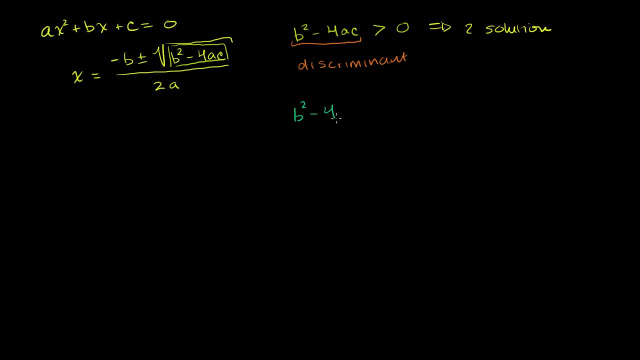 Now what happens if b squared minus 4ac is equal to 0?? So if this is equal to 0, if you take b squared minus 4 times a times c, and that's equal to 0, that tells us that this part of the quadratic formula is going to be 0, and the square root of 0 is just 0.. 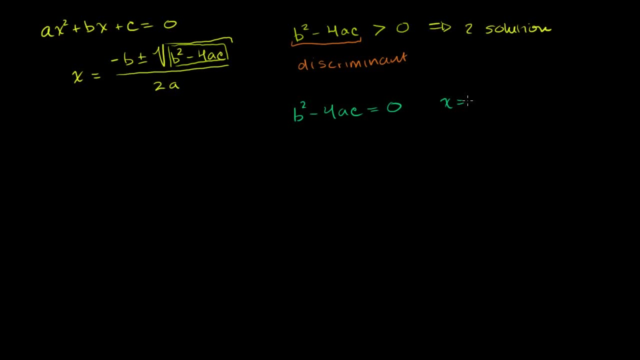 And then actually your only solution is going to be: x is going to be equal to negative b over 2a, Or another way to think about it is: you only have one solution. so if the discriminant is equal to 0, you only have one solution. 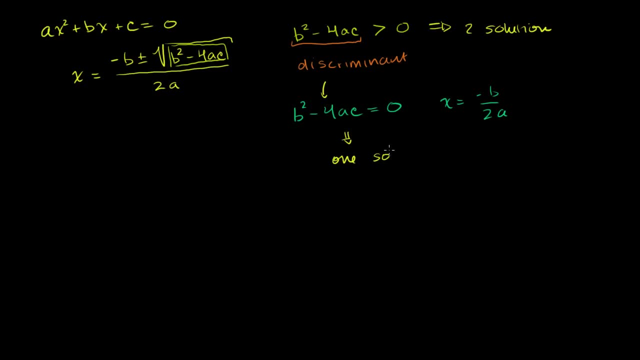 So if the discriminant is equal to 0,, you only have one solution. So if the discriminant is equal to 0, you only have one solution, one solution, and that solution is actually going to be the vertex, or the x-coordinate of the vertex. 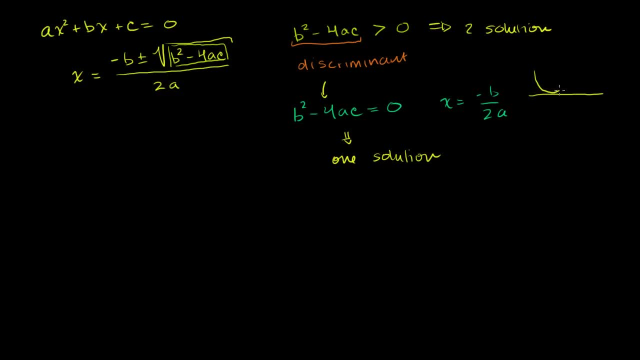 because you're going to have a parabola that just touches the x-axis, like that just touches there, or just touches, like that just touches at exactly one point when b squared minus 4ac is equal to 0. And then the last situation is if b squared minus 4ac, 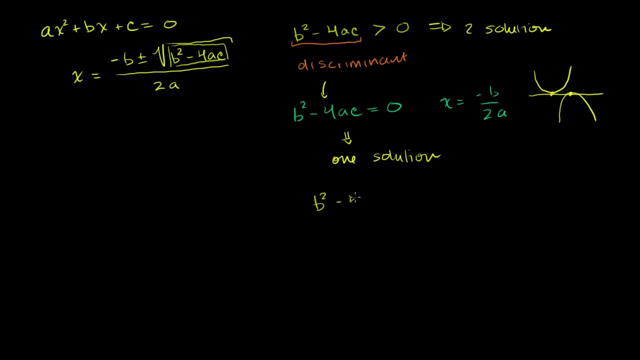 is less than 0.. b squared minus 4ac is less than 0. Then over here you're going to get a negative number under the radical- And we saw an example of that in the last video. And if we're dealing with real numbers, 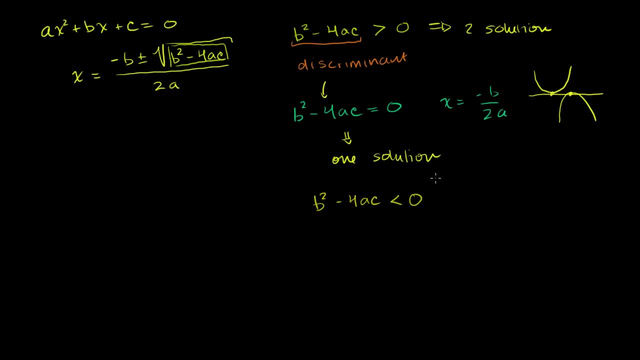 we can't take a square root of a negative number, So this means that we have no real solutions. In the future, you're going to see that we will have complex solutions, But if we're dealing with real numbers, we have no real solution because this: 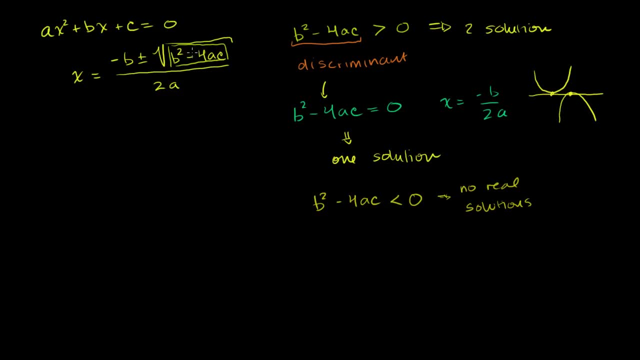 makes no sense Again, square root of a negative number, at least it makes no sense in the real numbers. And then there's more you can think about If we do have a positive discriminant. if b squared minus 4ac is positive. 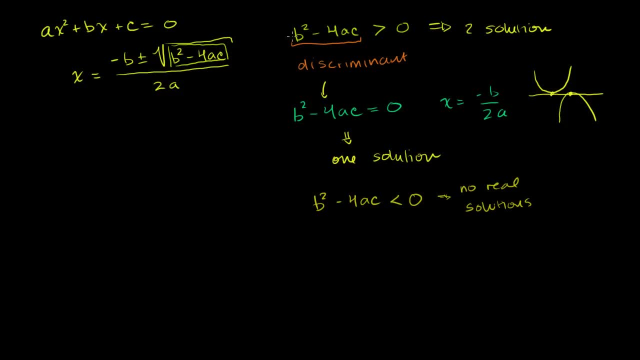 we can think about whether the solutions are going to be rational or not. If this is like 2, then we're going to have the square root of 2 in our answer. It's going to be an irrational answer or our solutions are going to be irrational. 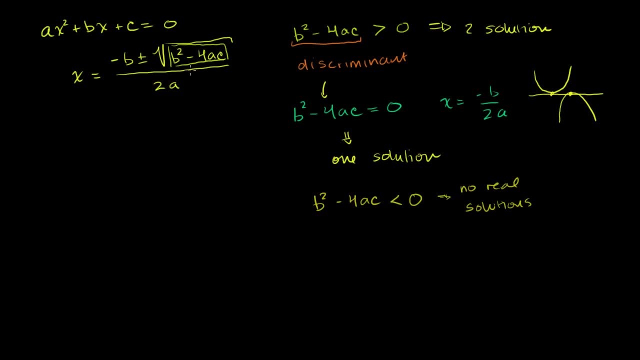 If b squared minus 4ac is 16, we know that's a perfect square. You take the square root of a perfect square. we're going to have a rational answer. Anyway, with all of that talk, let's do some examples. 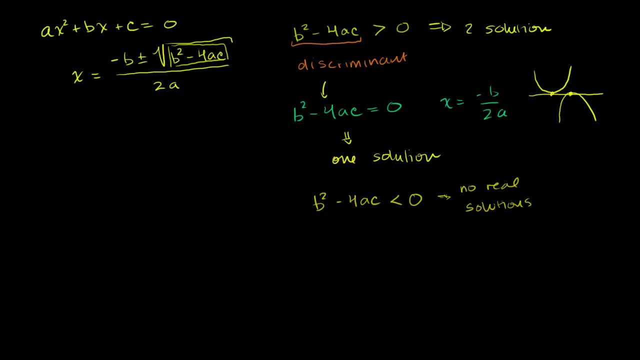 because I think that's what makes all of these ideas tangible. So let's say I have the equation: negative x squared plus 3x minus 6 is equal to 0.. And all I'm concerned about is: I just want to know a little bit about what kinds of solutions. 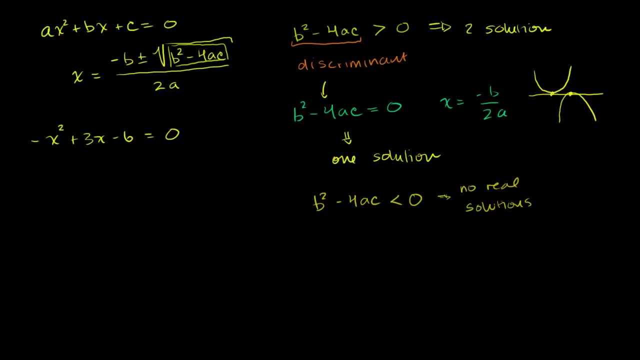 this has. I don't want to necessarily even solve for x. So if you're in a situation like that, I can just look at the discriminant. I can just look at b squared minus 4ac. So the discriminant here is what. 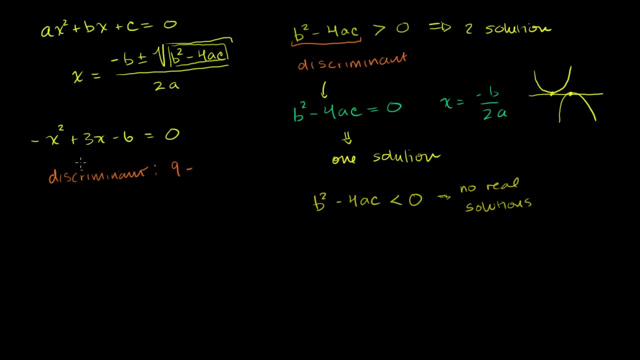 b squared is 9 minus 4 times a negative 1, times c, which is negative 6.. So what is this equal to This negative and that negative cancel out, but we still have that negative out there. So it's 9 minus 4 times 6.. 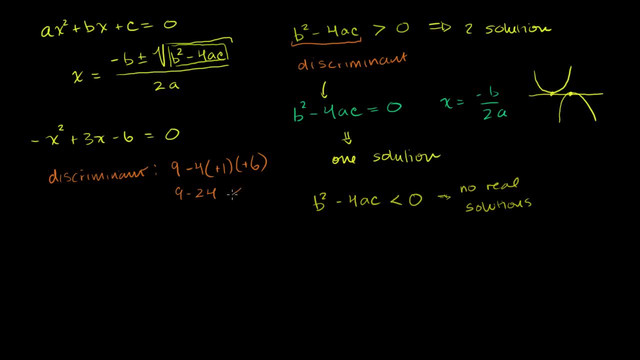 This is 9 minus 24, which is less than 0.. So we're going to have a number smaller than 0 under the radical. So we have no real solutions. That was this scenario right here, And so this graph is going to point downwards. 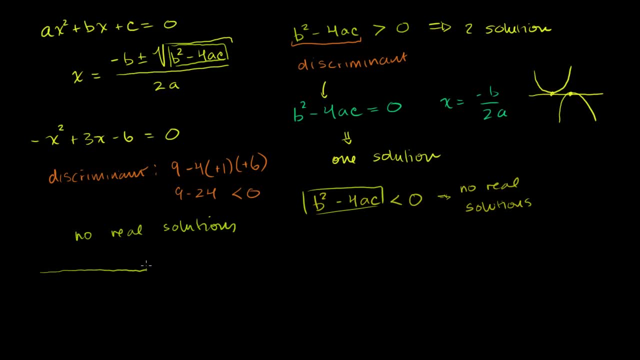 because we have a negative sign there. So it probably looks like something like that. If that's the x-axis, the graph is dipping down. Its vertex is below the x-axis at its downward opening, So it never intersects the x-axis. We have no real solutions. 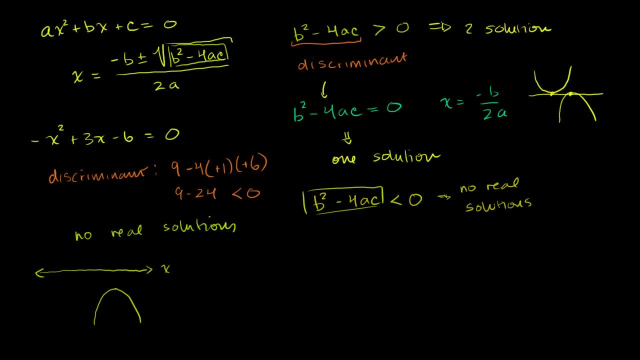 Let's do another one. Let's say I have. I'll do this one in pink. Let's say I have the equation 5x squared is equal to 6x. Well, let's put this in the form that we're used to. 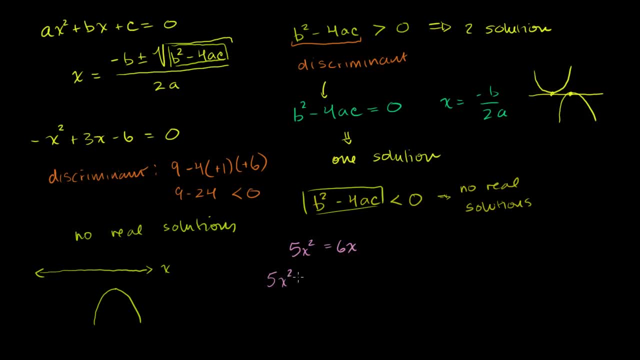 So let's subtract 6x from both sides And we get 5x. squared minus 6x is equal to 0.. And let's calculate the discriminant. So we want to get b squared. b squared is negative 6x. 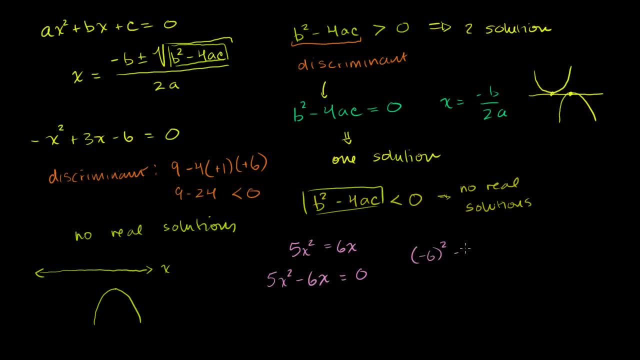 So negative 6 squared minus 4 times a times c. Well, where's the c? here? There is no c. here There's a plus 0 that I'm not writing. here There's no c. So in this situation c is equal to 0.. 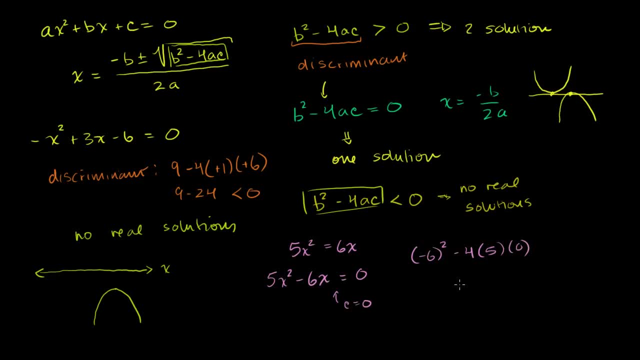 There is no c in that equation, So times 0.. So that all cancels out Negative. 6 squared is positive 36.. The discriminant is positive. You'd have a positive 36 under the radical right there. So not only is it positive, 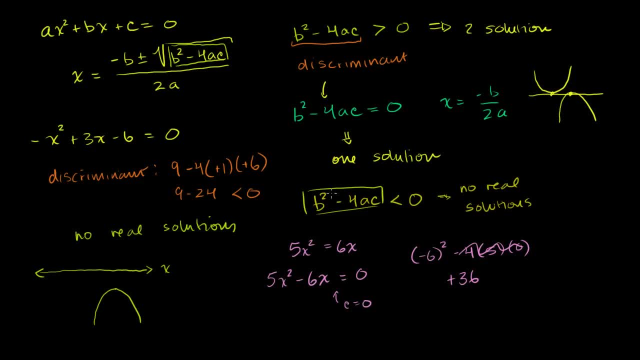 It's also a perfect square. So this tells me that I'm going to have two solutions. So I'm going to have two real solutions, And not only are they going to be real, but I also know they're going to be rational. 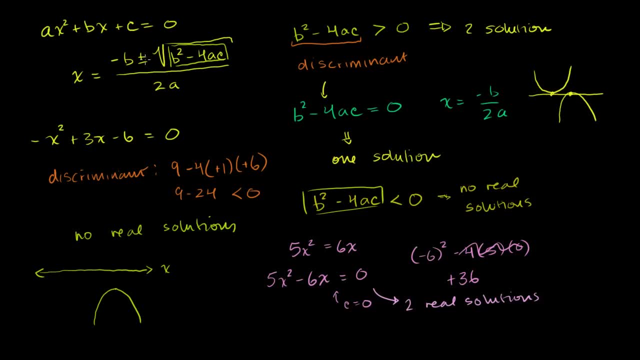 Because I have the square root of 36.. Square root of 36 is positive or negative 6. I don't get to end up with an irrational number here. So two real solutions that are also rational. This is this scenario, Right there. 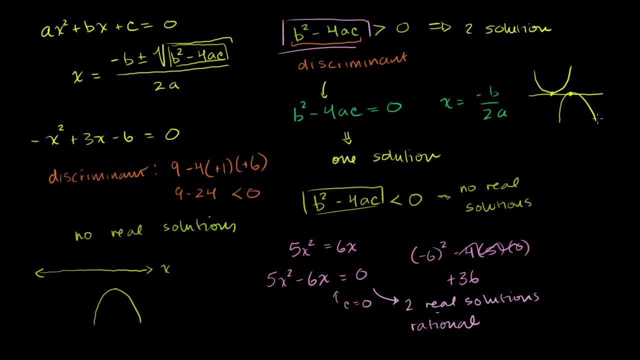 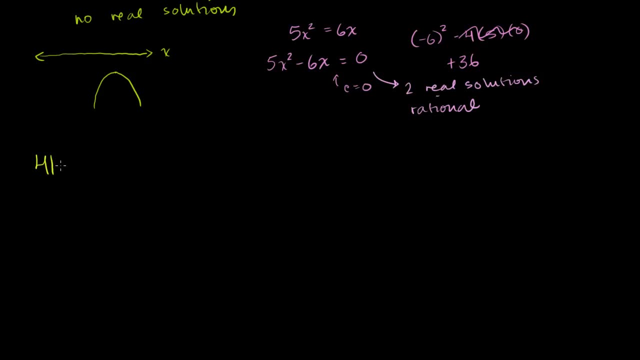 And you could also have irrational in this scenario. So it's this scenario plus the irrational. Let's do a couple more just to get really warmed up. Let's say I have 41x squared minus 31x minus 52 is equal to 0.. 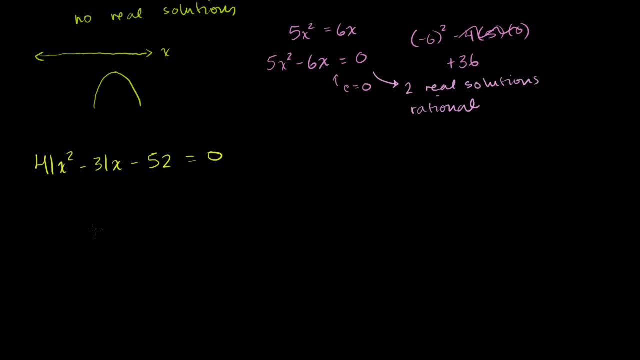 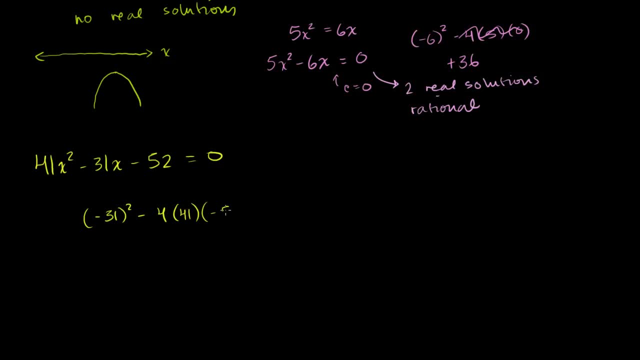 Times 41x. Times c Times: negative 52.. So what do I have here? This is going to be a positive 31 squared. The negative times the negative. these are both positive, So I'm going to have a positive. 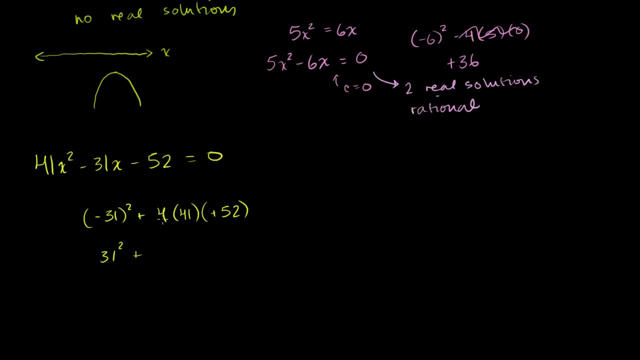 This is the same thing as 31 squared Plus. this is a positive number right here. I mean we could calculate it, but it's 4 times 41, times 52.. All I care about is my discriminant is positive. 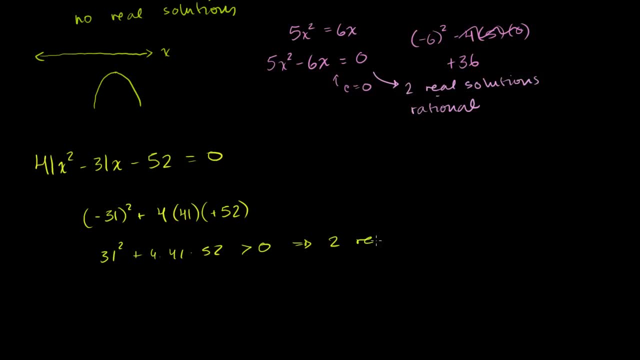 It is greater than 0.. So that means I have two real solutions And we could think about whether this is some type of perfect square. I don't know, I'm not going to do it here. That would take a little bit of computation. 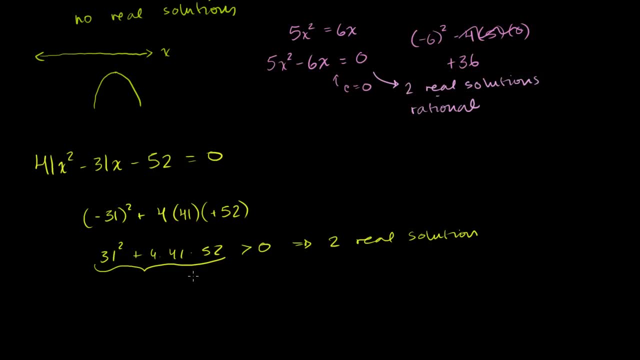 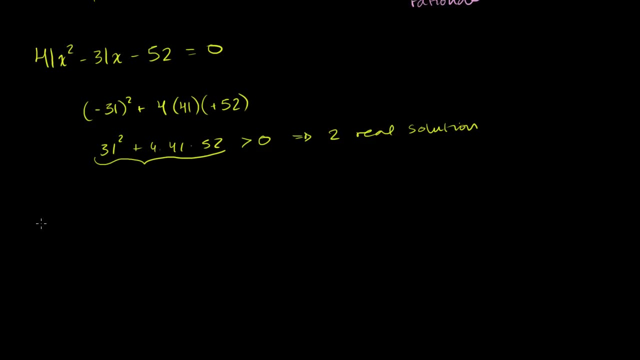 So we don't know if they're real or we don't know if they're rational or irrational solutions. Let's do one more of these. Let's say I have x squared minus 8x plus 16 is equal to 0.. Once again, let's look at the discriminant. 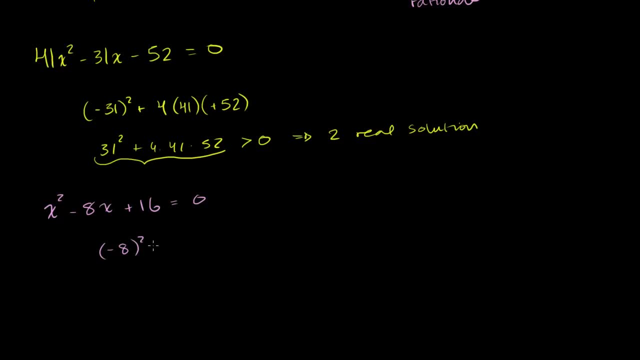 b squared, that's negative 8 squared minus 4 times a, which is 1, times c, which is 16.. This is equal to 64 minus 64, which is equal to 0. So we only have 1.. 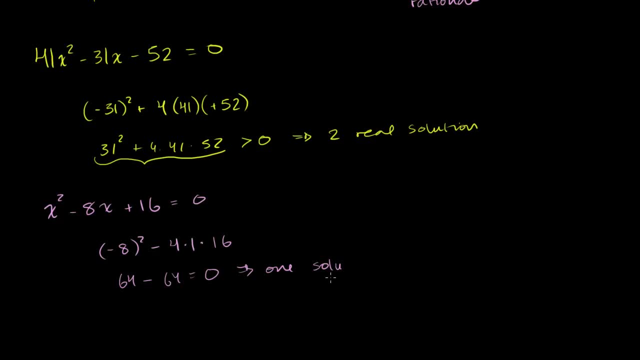 And by definition it's going to be rational. I mean, you could actually look at it right here. This is x minus 4 times x minus 4 is equal to 0.. The one solution is: x is equal to positive 4.. 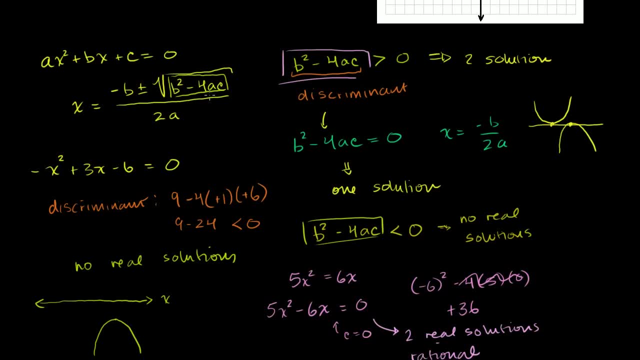 And when I say by definition of the quadratic formula, you look there, If this is 0, all you're left with is negative b over 2a, which is definitely going to be rational, assuming you have a, b and c are, of course, rational numbers. 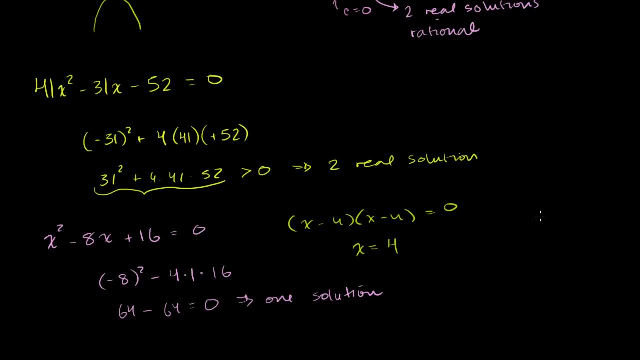 Anyway, hopefully you found that useful. It's a quick way if you don't have to go all the way to solving the solution. you just want to have to say what types of solutions or how many solutions, how many real solutions, or inspect whether they're real or rational.